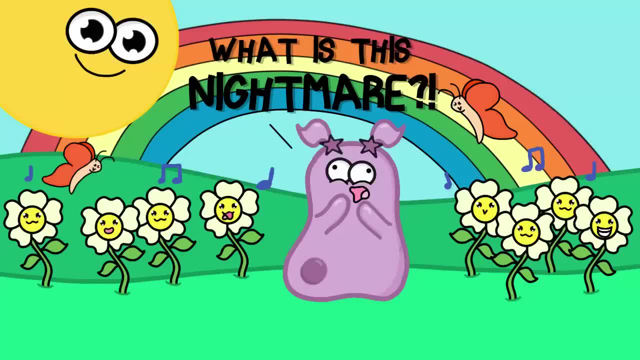 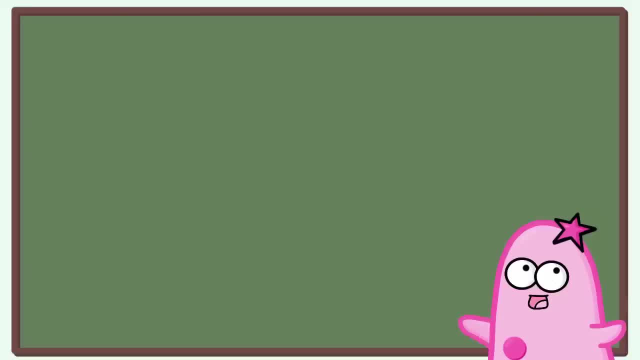 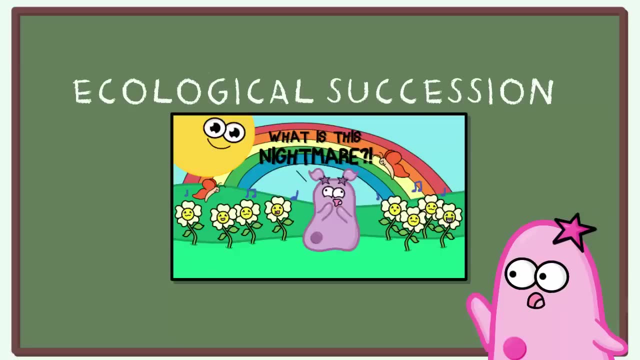 where they went, but they come back. You start seeing these small plants growing in where there hadn't been any plants for a while And, being a biology teacher, everything is destined to have a biology reference. So here's what it reminds me of Ecological succession. Although the movie 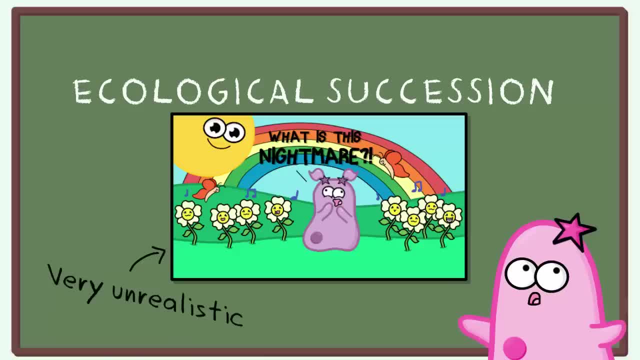 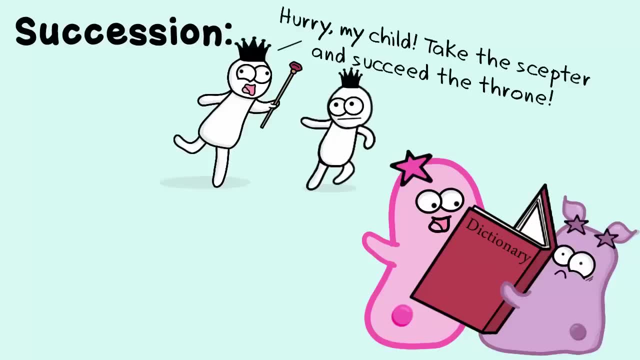 is kind of like an ultra-fast, impossible ecological succession. It's not really that fast in real life. Most dictionaries define succession as the following of a person or a thing after another in an order or a sequence. Well, ecological succession it's that, But in terms. 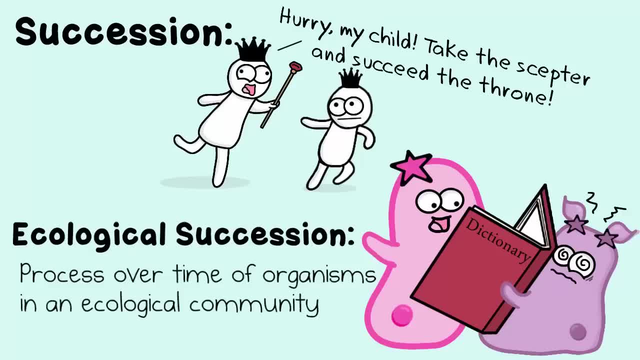 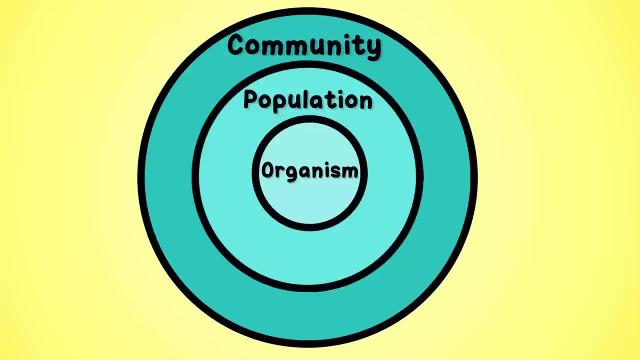 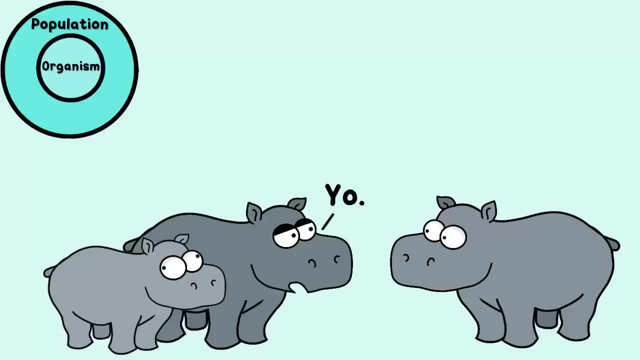 of ecology. ecological succession is a process over time of organisms in an ecological community. So what's a community? Well, in ecology we have different levels of organization. We have a living organism as our first level, like a hippo, And then we have a population. 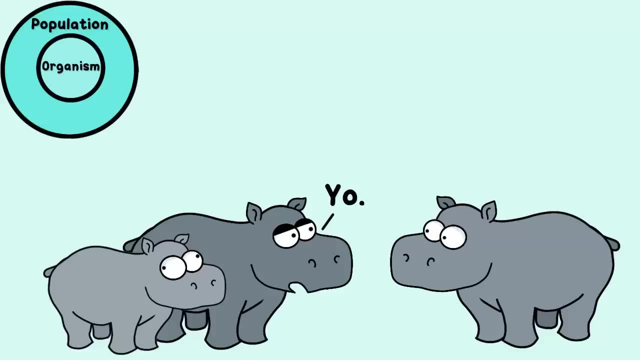 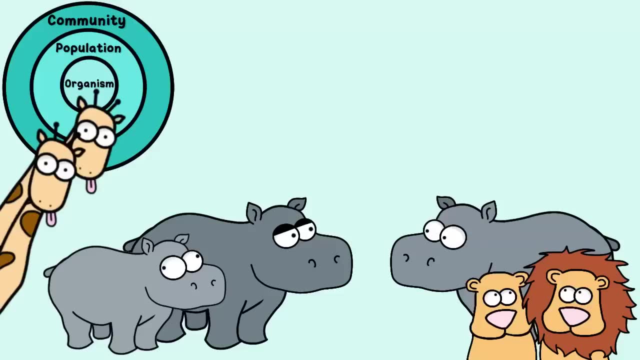 which is when you have the same species of an organism in a given area, So for example, a population of hippos, Same species, so that's one population, And then we have a community. It can involve many populations living together in an area. So now we have hippos, lions. 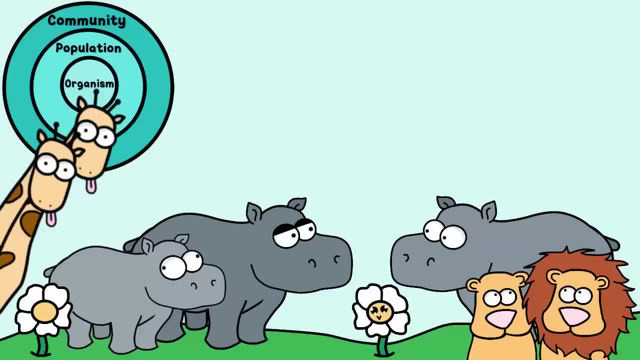 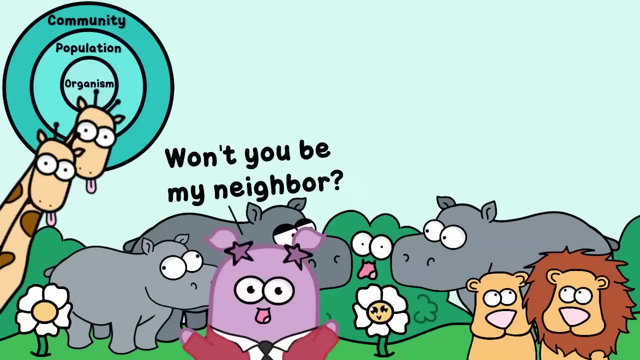 giraffes, And don't forget plants, because they can be a population too: Trees and shrubs. Now there are more levels beyond the community level, but this is our focus right now. Now there are two types of succession that we're going to briefly talk about. 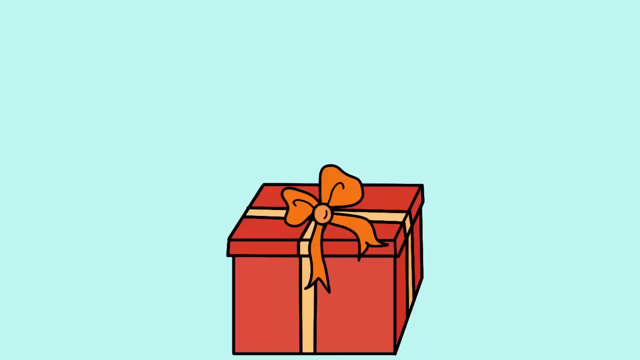 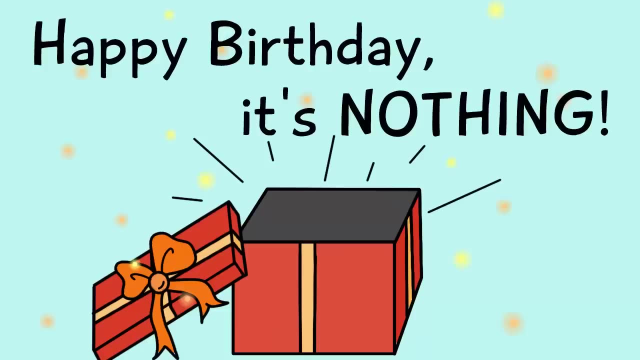 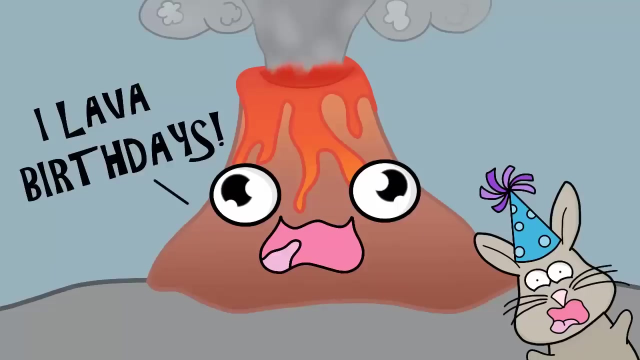 One is called primary succession. In primary succession, the area that this is happening to is brand new, at least in the sense that you're usually talking about an area that it doesn't have any soil, So this usually has to be a special circumstance. An example could be: 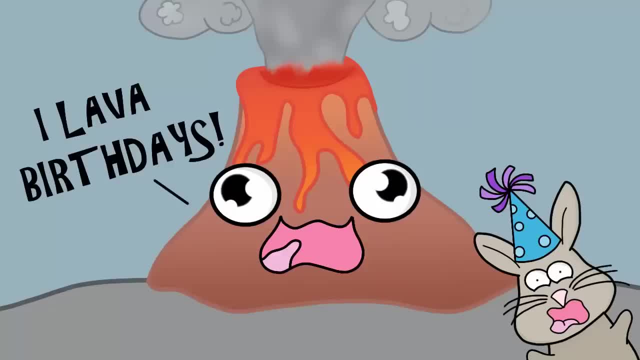 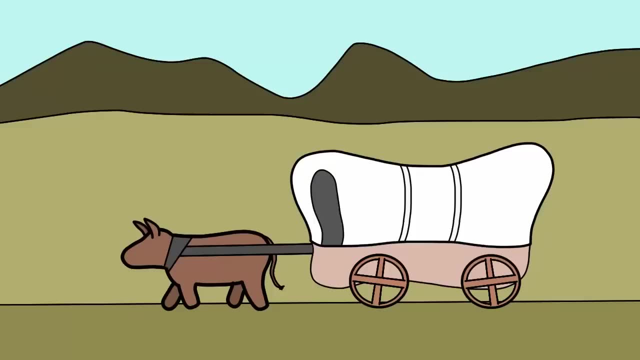 a volcano, lava flow that now has left this new area with no soil present, And usually you have a pioneer species, which that's the name for species that will colonize the area first. It sounds kind of exciting. Pioneer species and primary succession- Well, they can be organisms. 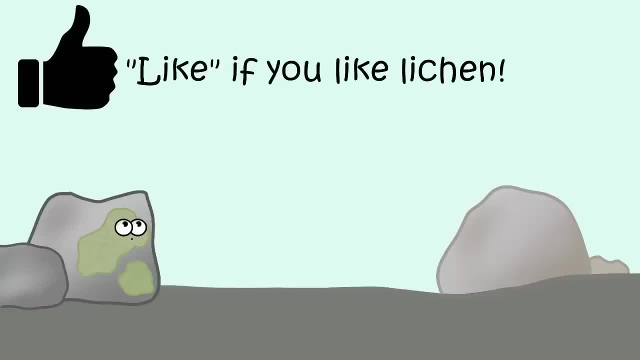 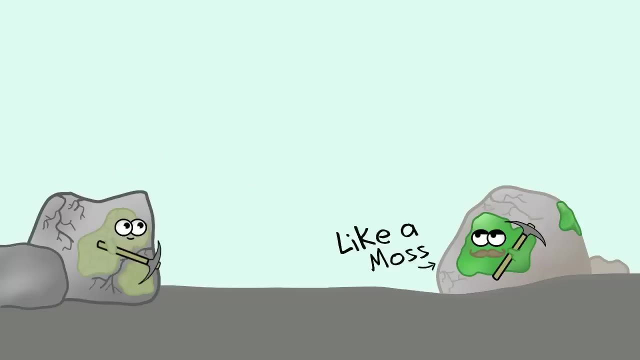 like lichen. If you're unsure about what lichen is, you need to Google it. It's likely you've seen lichen before. Moss is another potential pioneer. After pioneer, species colonize the area, they slowly break down rock into smaller, more plant-friendly substrate And, over time, 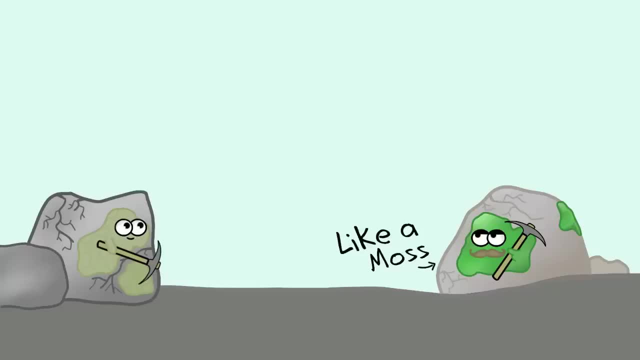 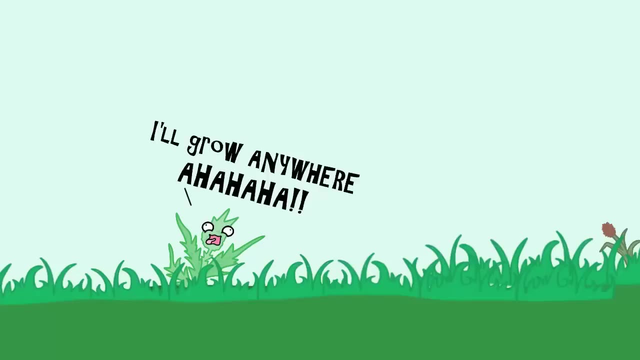 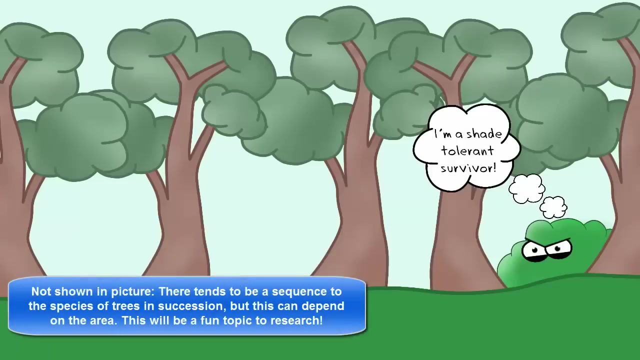 they can contribute more organic matter in this newly formed soil, which will help support all kinds of plants: Small vascular plants like grasses, and plants that you might consider weeds. Those will come in, and shrubs can follow, and then trees. All this time, animals can be moving into the area, And how long this takes it can vary. It's often 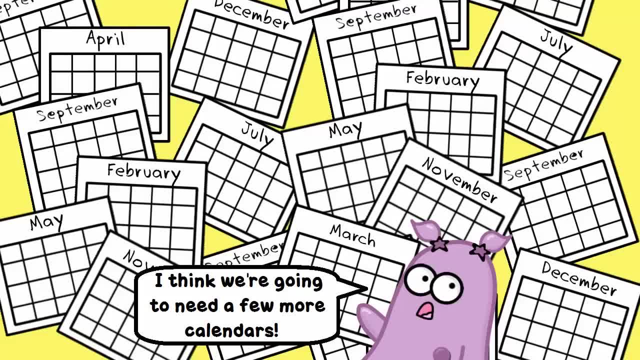 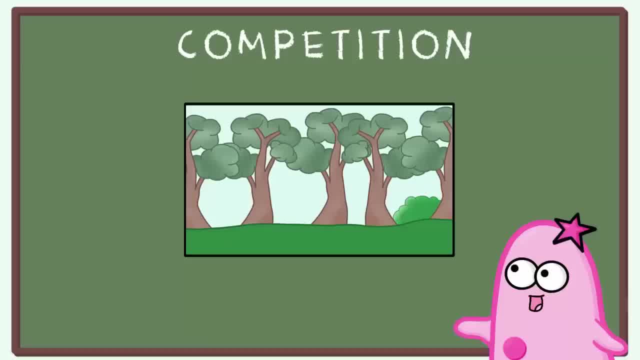 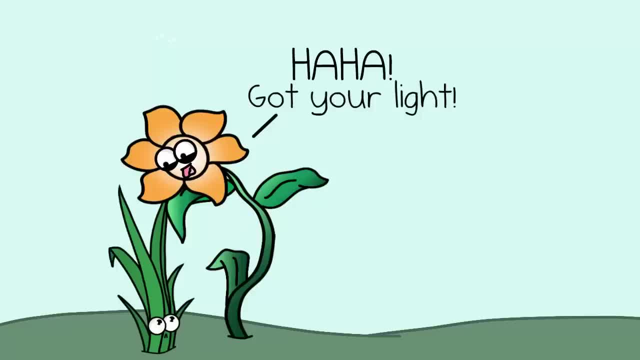 hundreds of years before you get your full climax community going. And if you're wondering, why this sequence with the plants? Why doesn't it just stop with the grass? Well, keep in mind that as other plants come in, these bigger plants, you're going to start to see more competition for space and resources. I mean think. 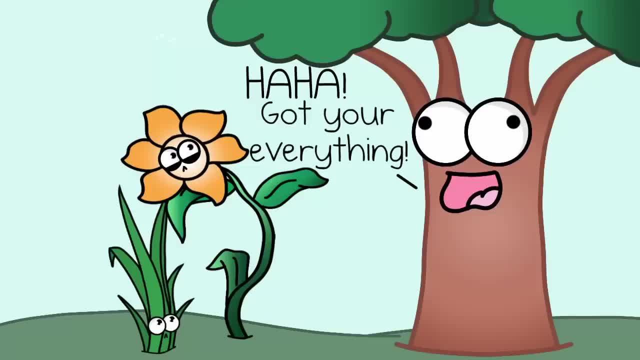 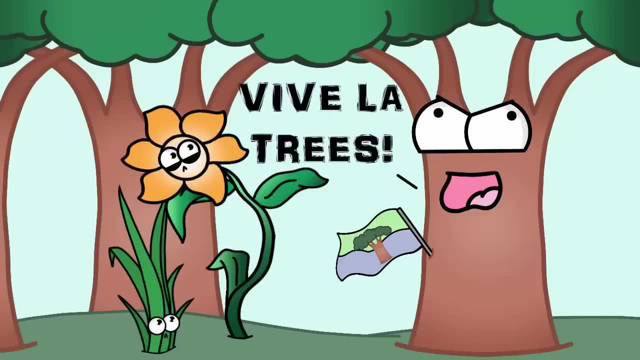 about how, how it would be by the time trees come in. As the trees grow larger, they could block some of the light that small plants underneath them might be dependent on. And as new, larger plant species come in, this competition can bring about a new order. 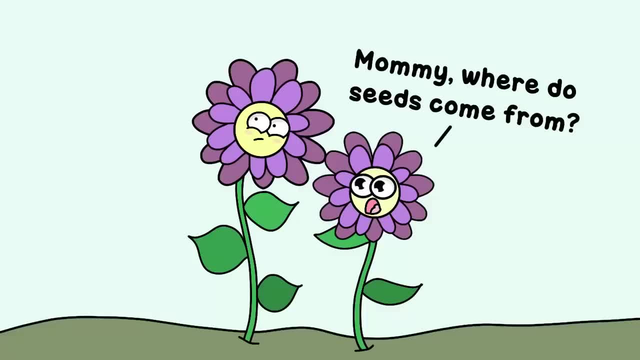 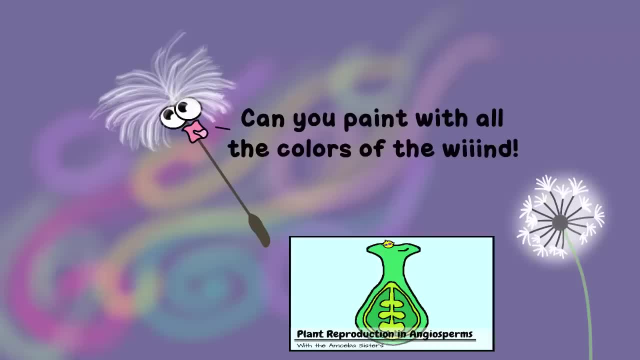 And if you're wondering, where did these plants even come from? Well, there's so many ways that seeds can be dispersed: wind, water, animals. Check out our plant reproduction video for more information about how these plants could actually have come into the area. 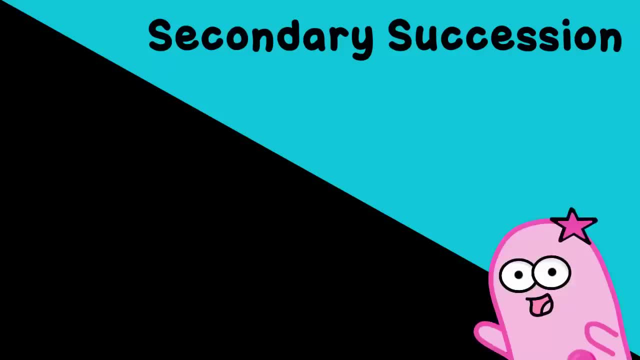 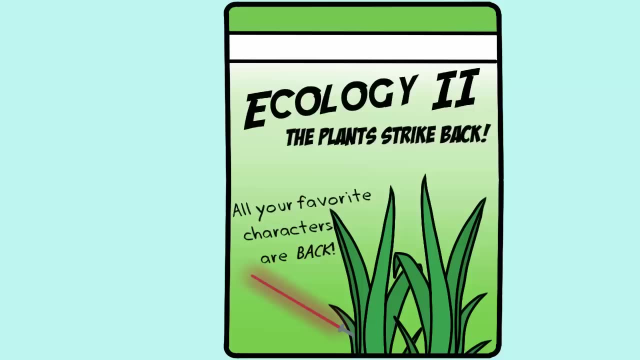 Now for secondary succession. Similar to primary succession, it follows a typical ecological sequence. With secondary succession I like to think second, because it's like coming back again a second time. And what I mean by that is it's usually you're talking about an area. 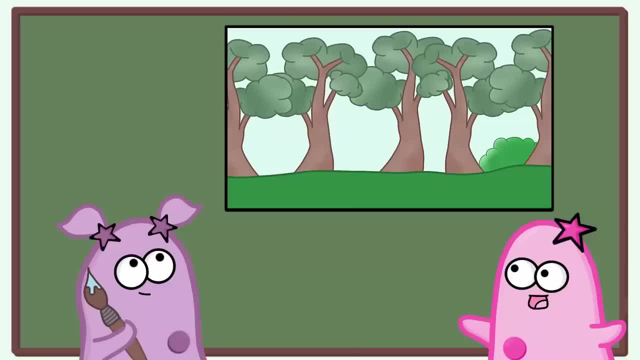 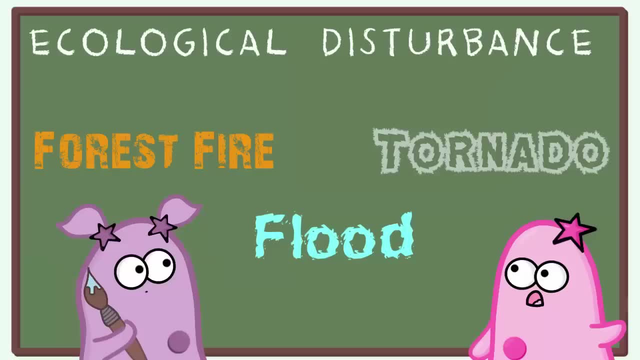 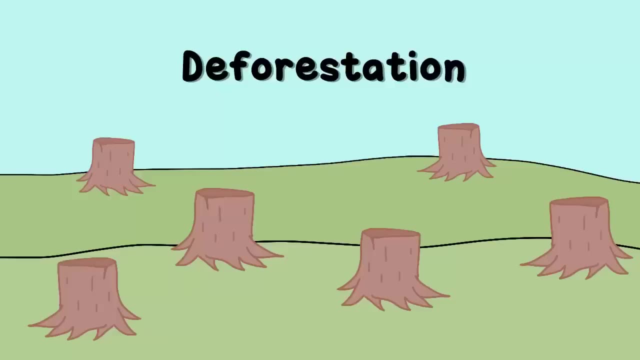 that once had plants and animals and a full ecological community going on, but then you had a disturbance, an ecological disturbance, like a forest fire or a flood, a tornado. Actually, it doesn't even have to be a natural disaster. Human activity can be involved with secondary succession too. 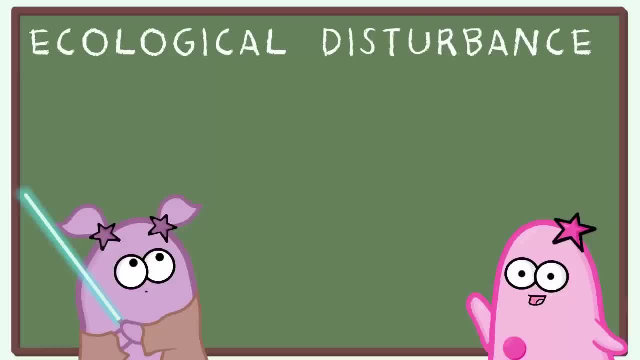 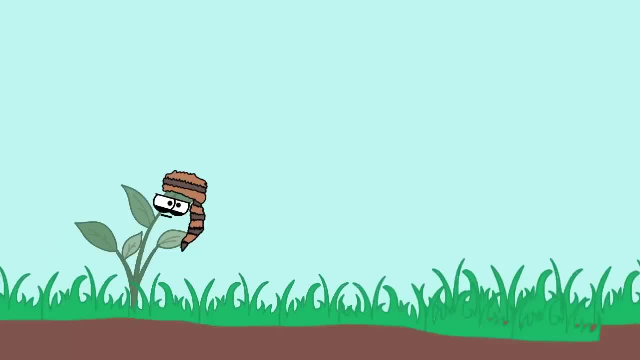 Regardless of the type of event in secondary succession the soil is still there, And so that's kind of a big key point here, because you actually have soil to grow in So you don't have to have this really hardy pioneer species because in secondary succession